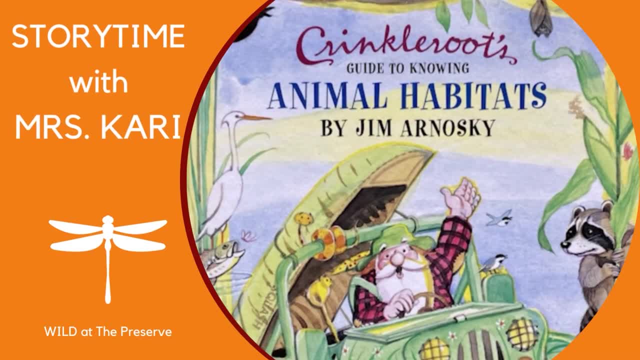 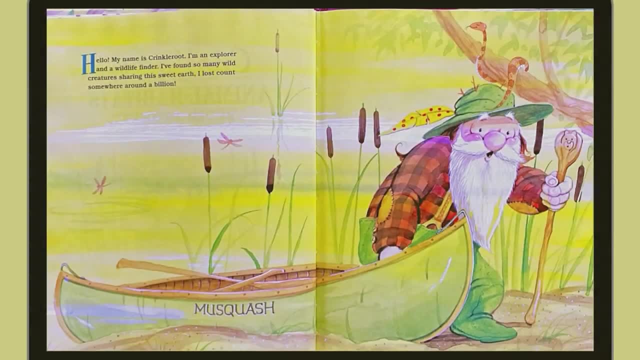 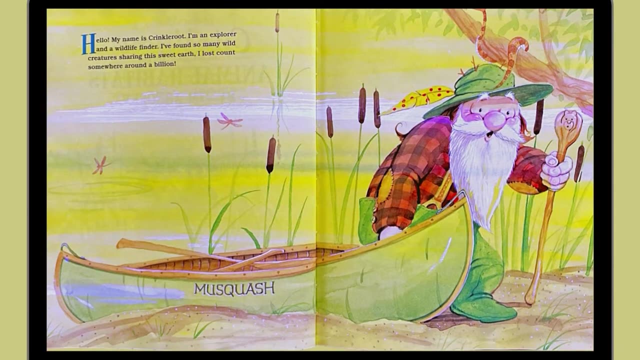 Crinkle Root's Guide to Knowing Animal Habitats by Jim Arnowski. Hello, my name is Crinkle Root. I'm an explorer and a wildlife finder. I found so many wild creatures sharing this sweet earth- I lost count- somewhere around a billion. 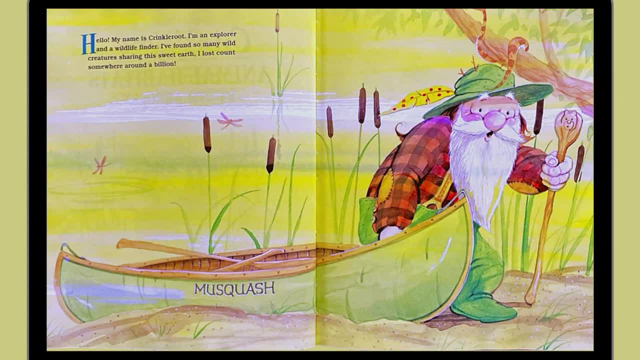 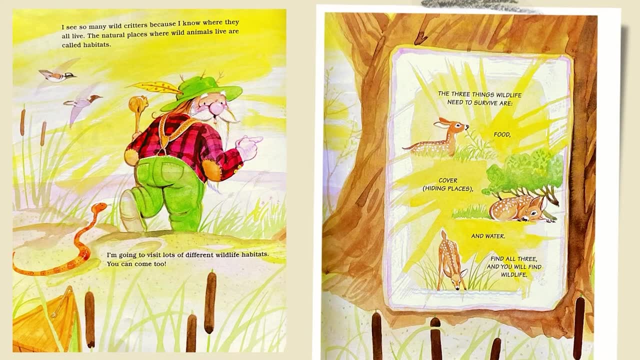 I see so many wild critters because I know where they all live. The natural places where wild animals live are called habitats. I'm going to visit lots of different wildlife habitats. You can come too. The three things wildlife need to survive are food, a cover, or shelter and water. 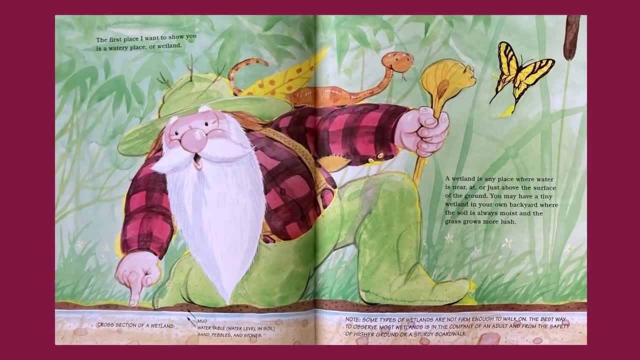 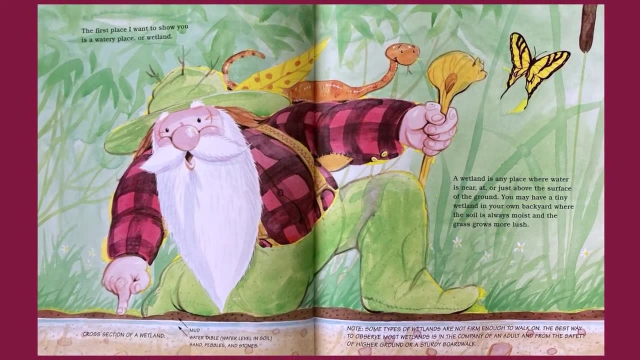 If you find all three, you will find wildlife. The first place I want to show you is a watery place, or a wetland. A wetland is any place where water is near at or just above the surface of the ground. You may have a tiny wetland in your home. You may have a tiny wetland in your own backyard, where the soil is always moist and the grass grows more lush. The three most common wetlands are marshes, swamps and bogs. 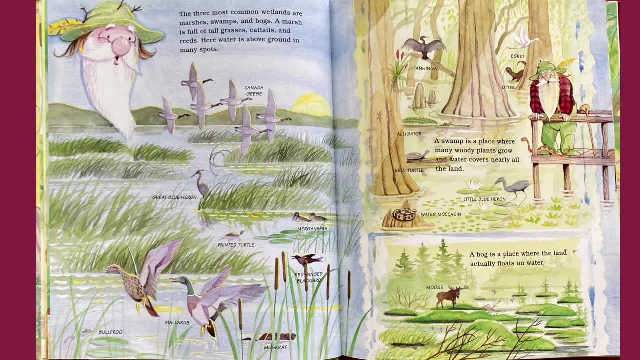 A marsh is full of tall grasses, cattails and reeds. Here, water is above ground in many spots. A swamp is a place where many wooded plants grow and water covers nearly all the land. A bog is a place where the land actually floats on water. 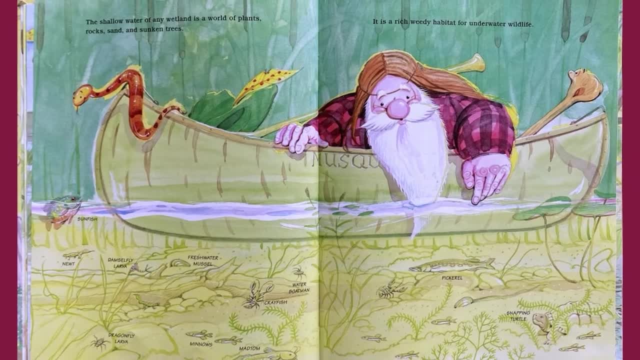 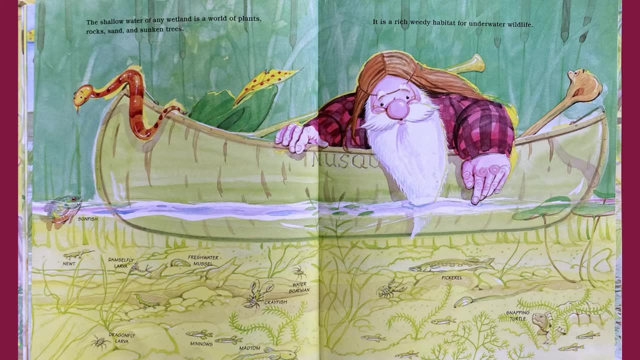 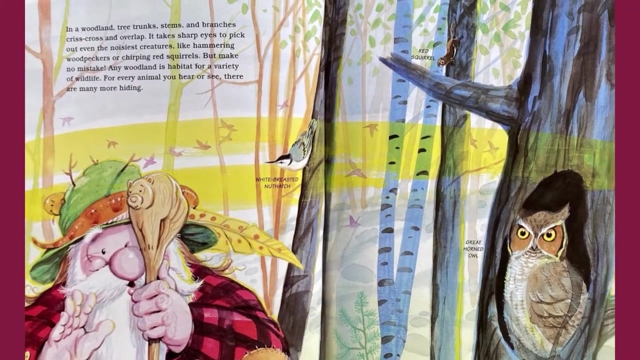 The shallow water of any wetland is a world of plants, rocks, sand and sunken trees. It is a rich, weedy habitat for underwater wildlife. In a woodland, tree, trunks, stems and branches criss-cross and overlap. 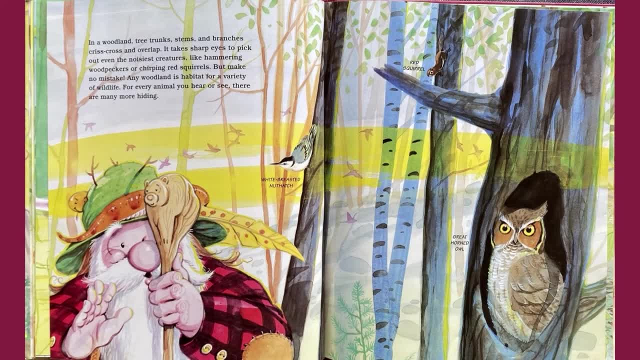 It takes sharp eyes to pick out even the noise, Even the noisiest creatures, like hammering woodpeckers or chirping red squirrels. But make no mistake, any woodland is a habitat for a variety of wildlife. For every animal you hear or see, there are many more hiding. 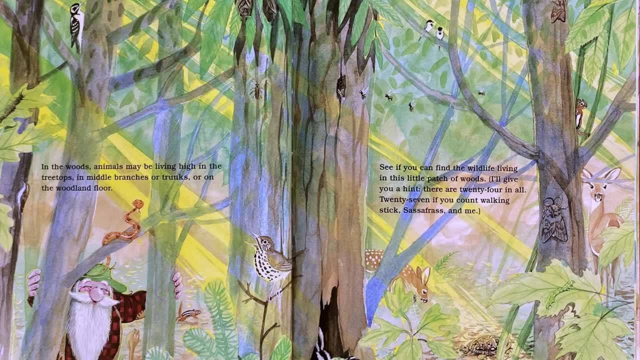 In the woods. animals may be living high or in the treetops, in middle branches or trunks or on the woodland floor. See if you can find the wildlife living in this little patch of woods. Climb aboard my old jalopy. 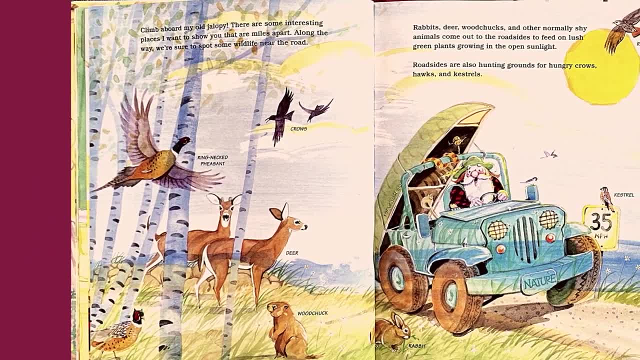 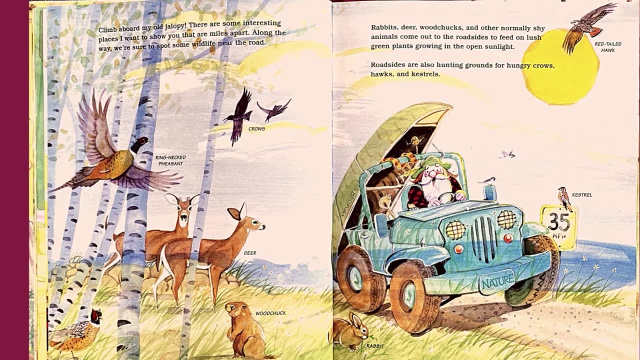 There are some interesting places I want to show you that are miles apart. Along the way, we're sure to spot some wildlife near the road. Rabbits, deer, woodchuck and other normally shy animals come out to the roadsides to feed on lush green plants growing in the open sunlight. 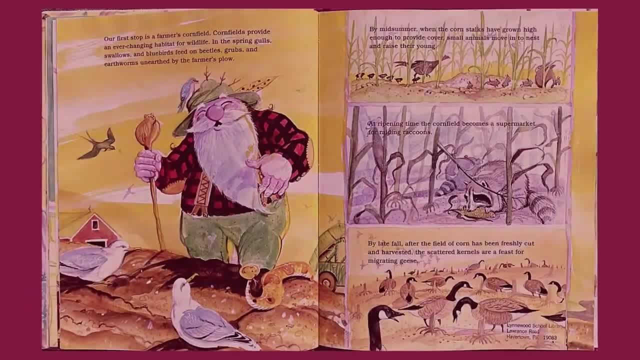 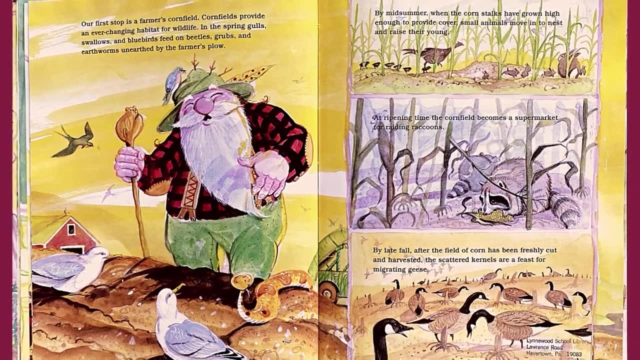 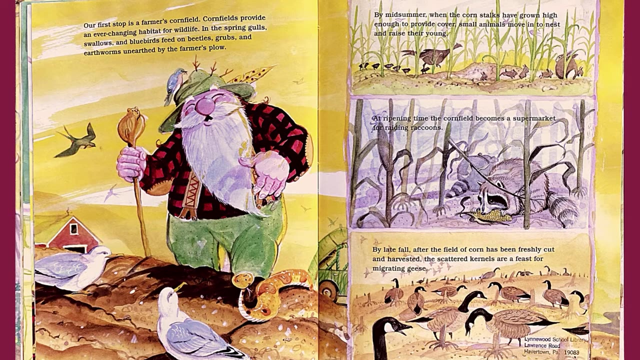 Roadsides are also hunting grounds for hungry crows, hawks and kestrels. Our first stop is a farmer's cornfield. Cornfields provide an ever-changing habitat for wildlife. In the spring, gulls, swallows and bluebirds feed on beetles, grubs and earthworms. underneath, unearthed by the farmer's plow. 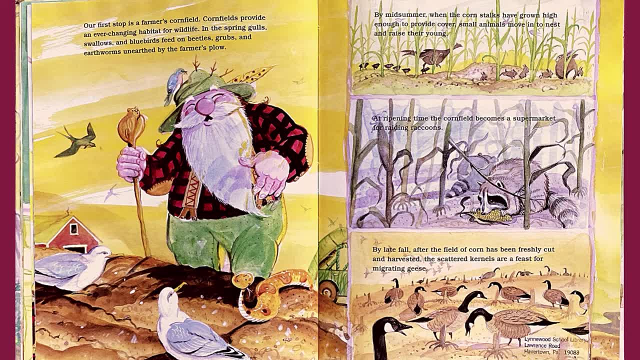 By mid-summer, when the corn stalks have grown high enough to provide cover, small animals move into the nest and raise their young. At ripening time, the cornfield becomes a supermarket for raiding raccoons. By late fall, after the field of corn has been freshly cut and harvested, the scattered kernels are a feast for migrating geese. 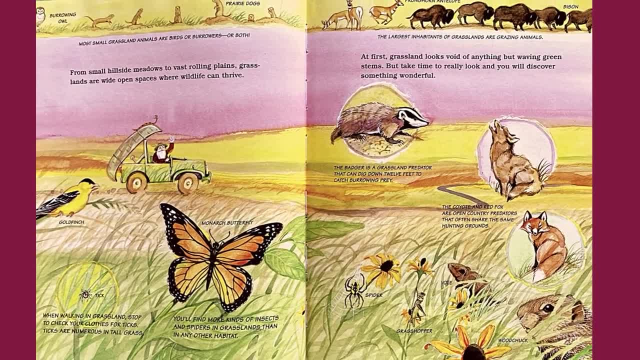 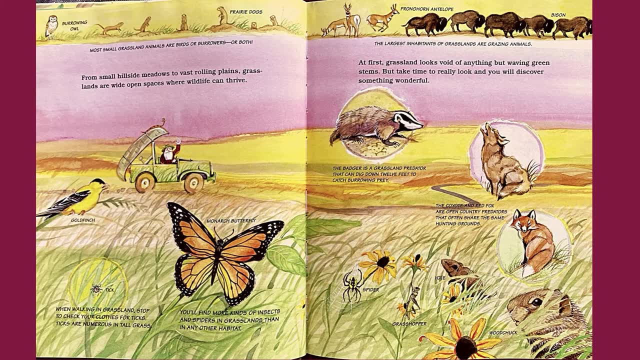 From small hillside meadow to vast rolling plains, grasslands are wide open spaces for animals. This is where wildlife can thrive. At first glance, grasslands look void of anything but waving green stems, But take a look, a good look, and you will discover something wonderful. 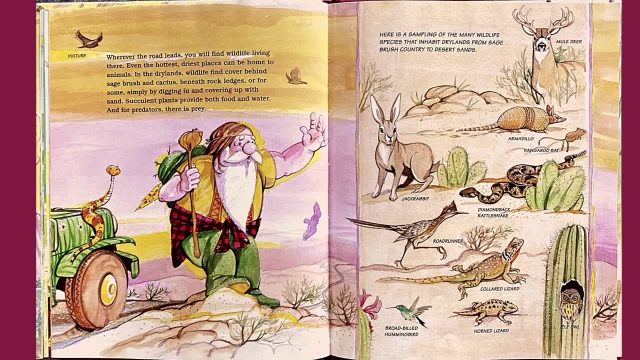 Wherever the road leads, you will find wildlife living there. Even the hottest, driest places can be home to animals. In the drylands, wildlife find cover behind sagebrush and cactus. They can be found on rock ledges or, for some, simply by digging in and covering up with sand. 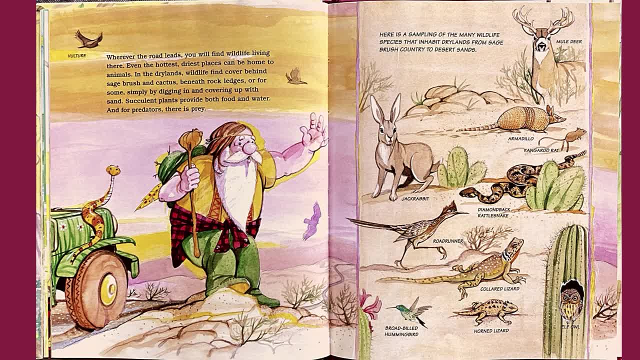 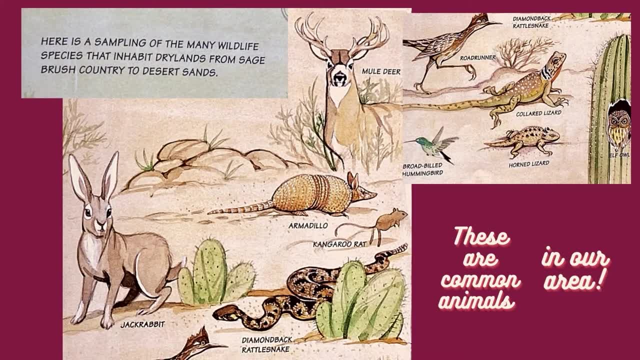 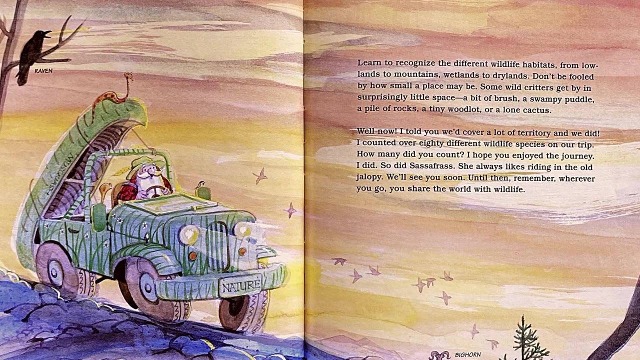 Succulent plants provide both food and water, And for predators there is prey. Here is a sampling of the many wildlife species that inhabit drylands, from sagebrush country to desert sands. Learn to recognize the different wildlife habitats, from lowlands to mountains, wetlands to drylands.